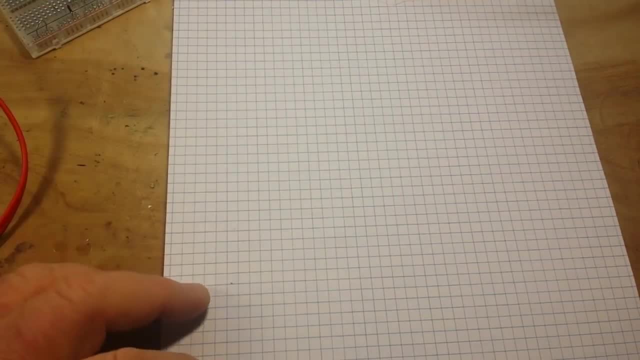 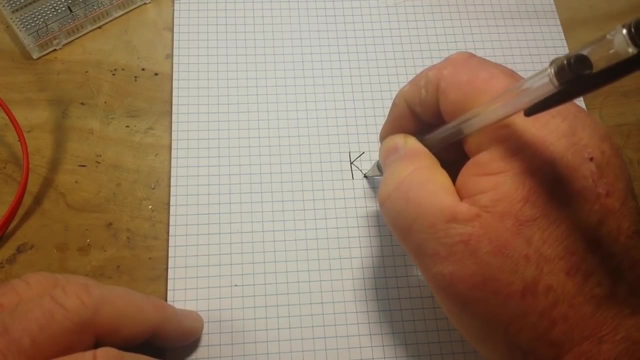 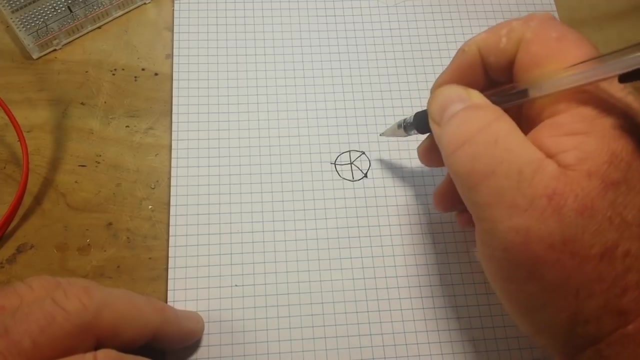 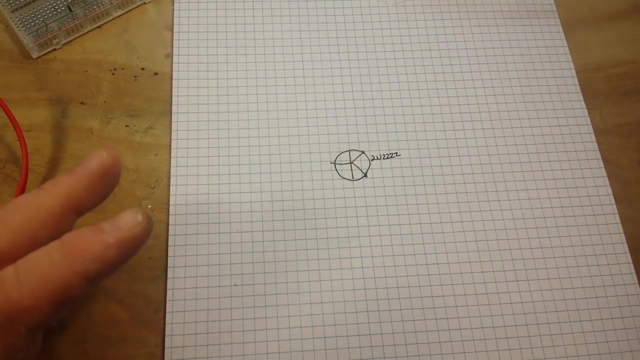 we're going to take a look at the operation. So first let's go over the common emitter amplifier. At the heart of it is an NPN transistor. For our purposes today, we're going to use the 2N2222.. It's just a simple transistor that's everywhere and it works well for small. 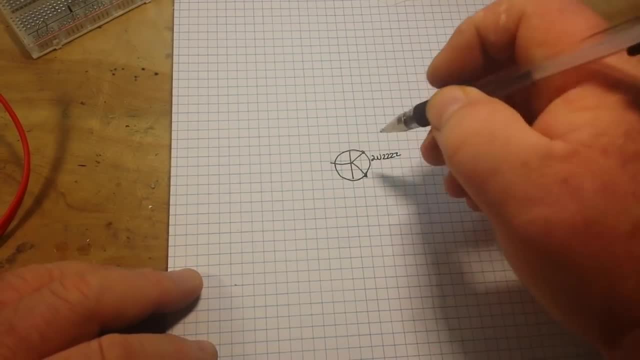 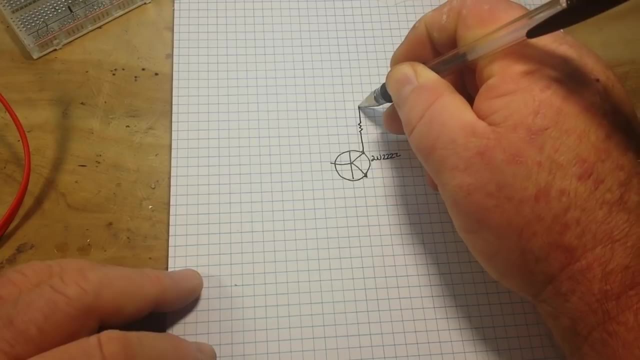 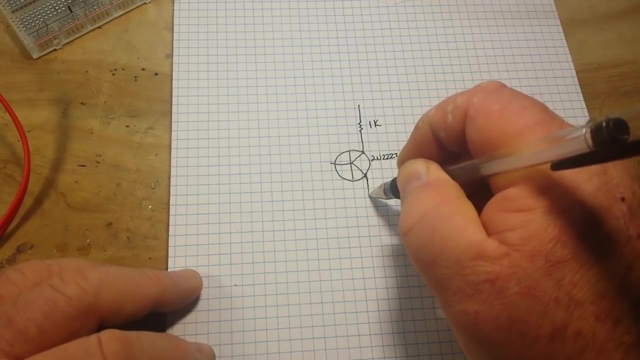 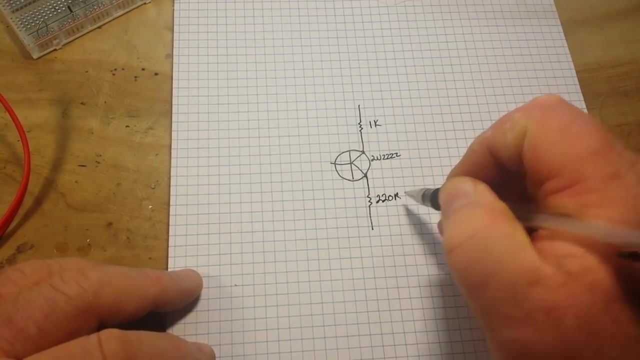 signal amplification like this. So we're going to start out From our collector through a collector resistor- In this case I'm going to use 1K- And then our emitter is going to have the emitter resistor, In this case 220 ohms. Now, remember the point. 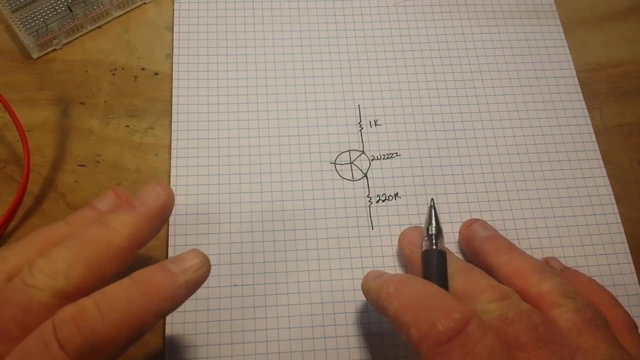 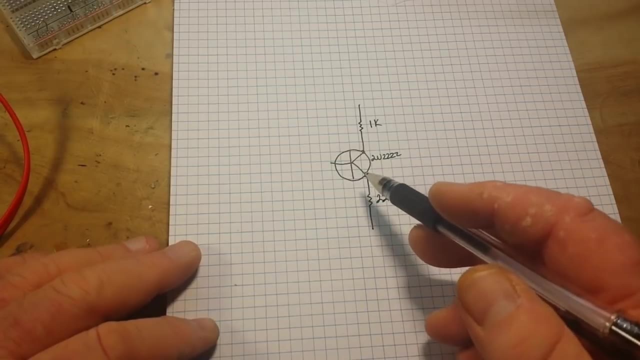 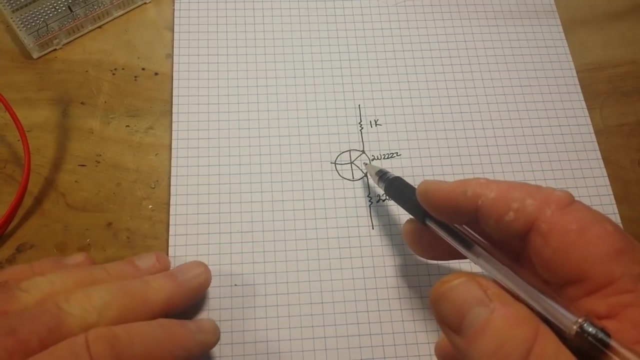 of the emitter resistor is to present, prevent, not to present to prevent a thermal runaway. Because what happens when you're doing this class A amplification is the harder the transistor drives, the hotter it gets, And the hotter it gets, the harder it can drive, So it gets. 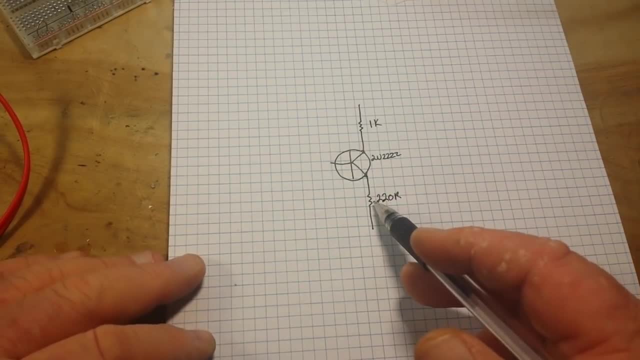 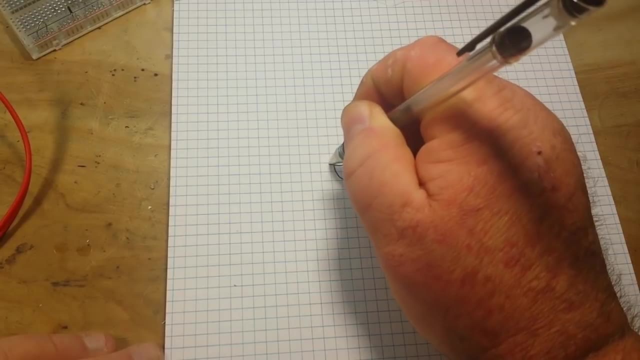 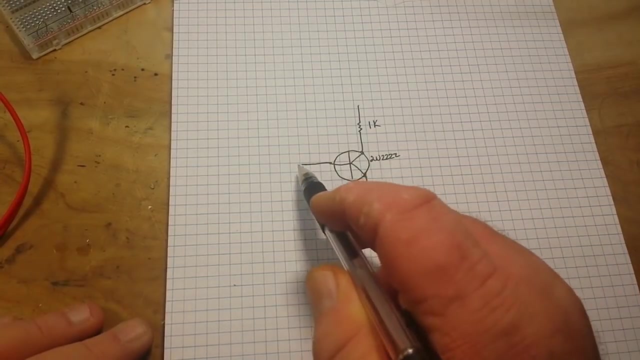 into this vicious loop where it will just burn itself out. So we just limit the amplification here with a resistor. Next, our signal comes in through the base, And that's the basics. The signal comes in through the base. It creates a larger current flow from the collector to 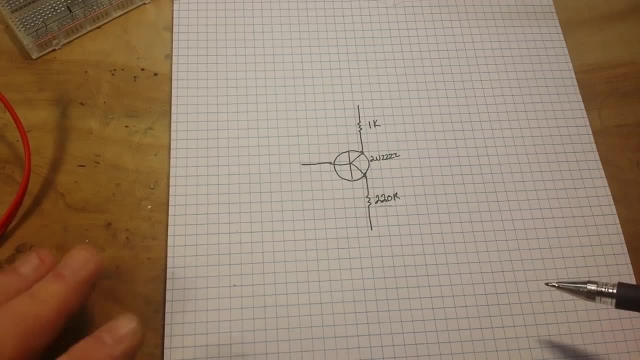 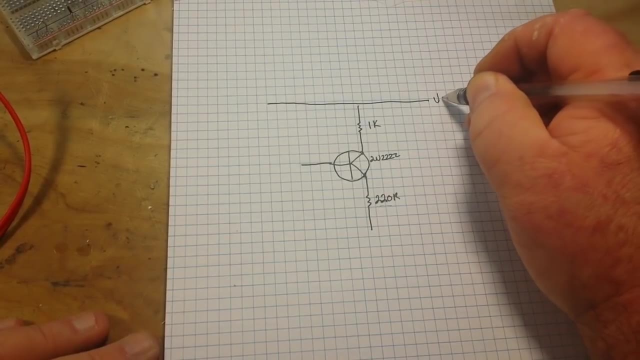 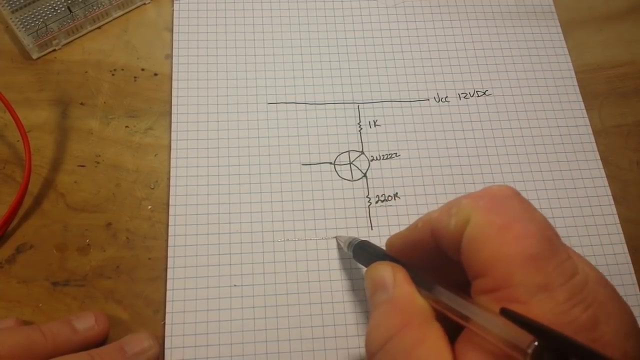 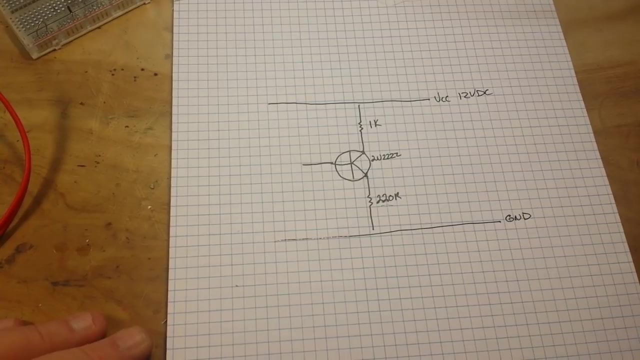 emitter junction And that's where our amplification comes from. So let's have our VCC up here And for our purposes, today it is going to be 12 volt DC And ground, of course, is down here. now the first thing that we want to do is we want to eliminate any dc coming into the circuit. 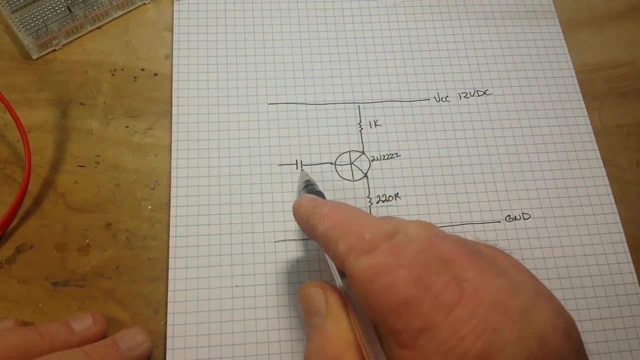 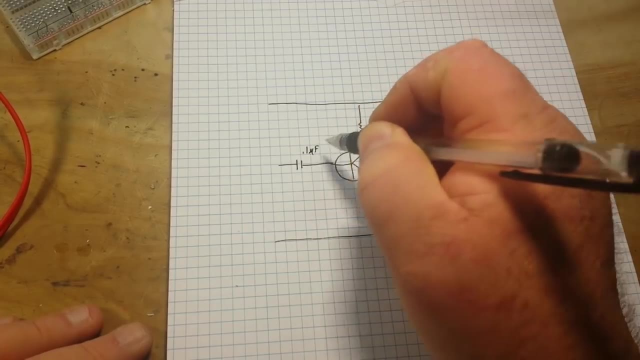 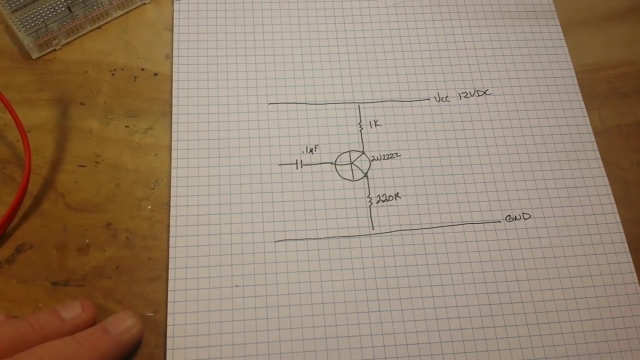 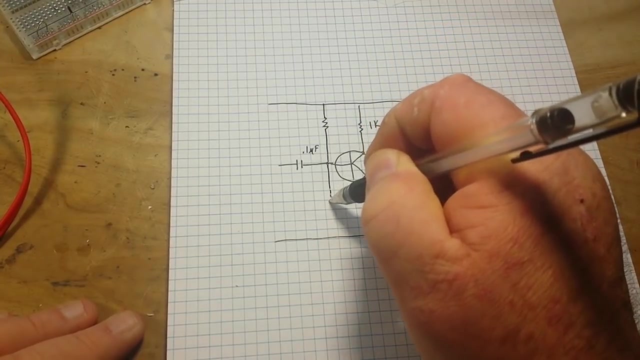 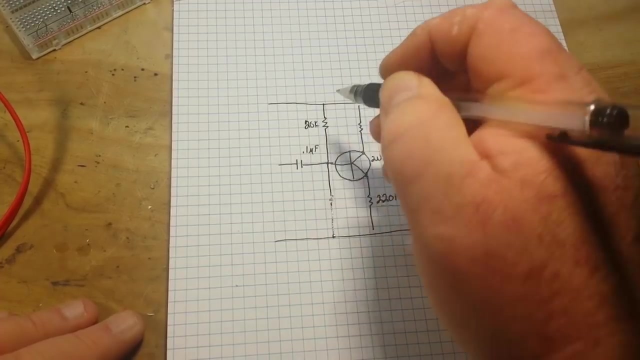 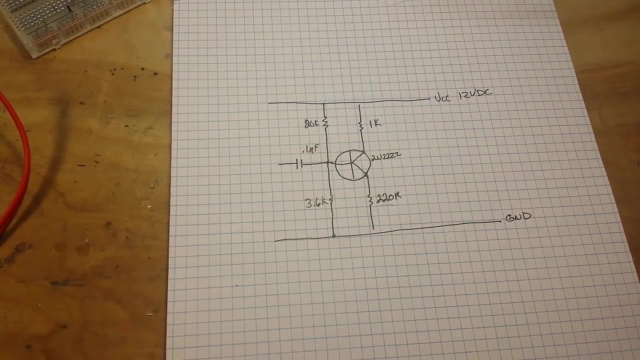 easy enough to do. we just put a capacitor on the input. i'm going to use 0.1. microfarad work just fine. now the next thing that we have to do is we have to bias the base of the transistor with a voltage divider. so two transistors. we're going to use 20k and 3.6k. i'm sure you remember. 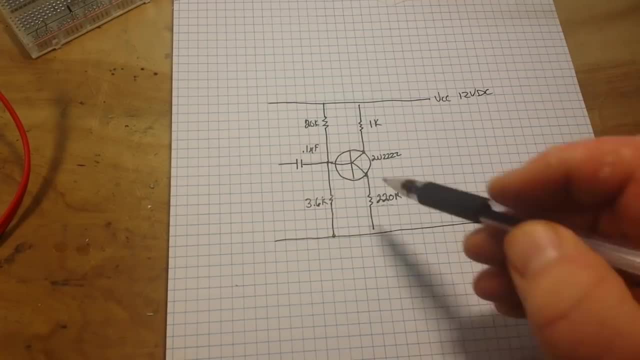 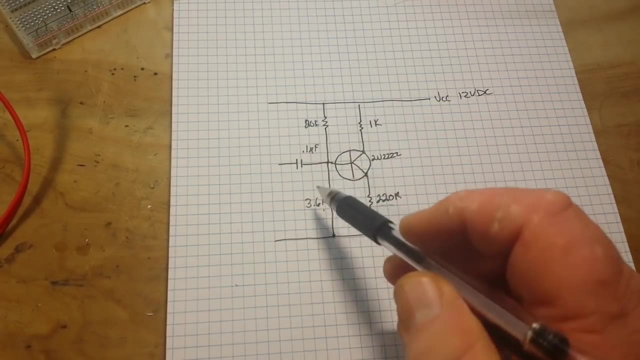 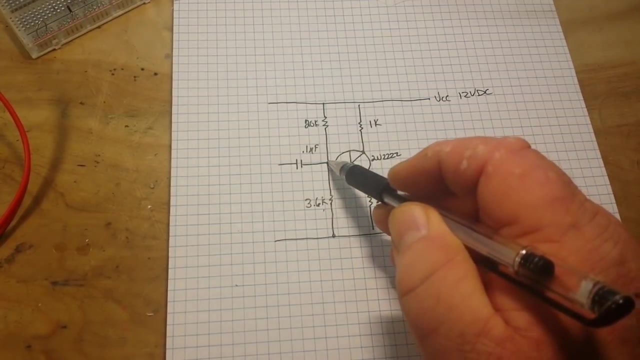 your voltage divider calculations but v out. so the voltage at this point here is r2 over r1 plus r2, and since we're doing 12 volts in this case, we're going to get about 1.8 volts here, and that is going to give us a nice bias point for our transistor. 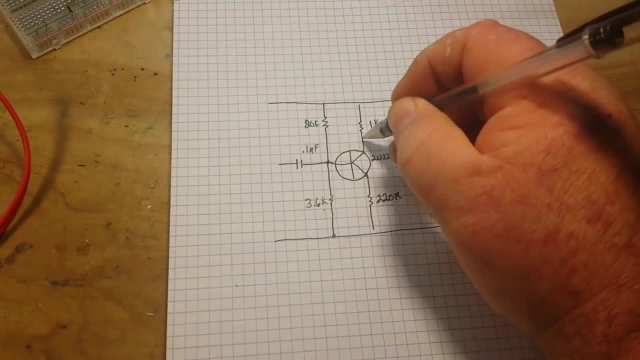 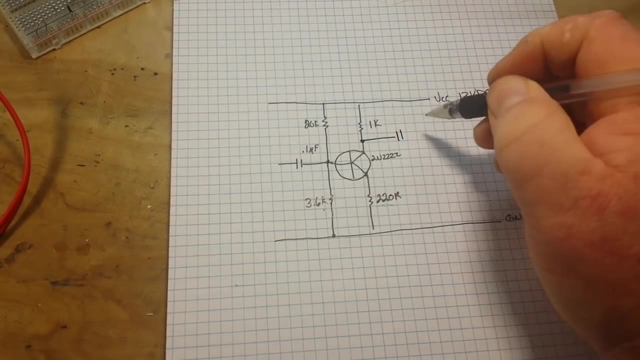 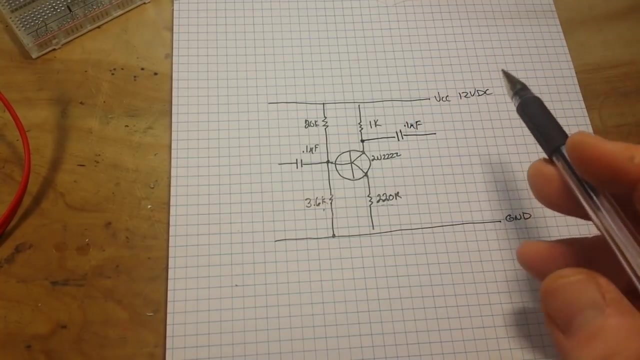 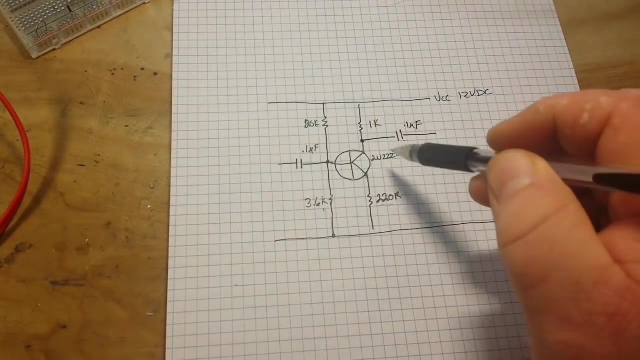 now we're going to take our output here off of the collector and again we want to eliminate any dc coming out, so we're going to use another 0.1 microfarad capacitor. so, and so we're blocking dc coming in, we're blocking dc coming out, so the only dc in the entire circuit. 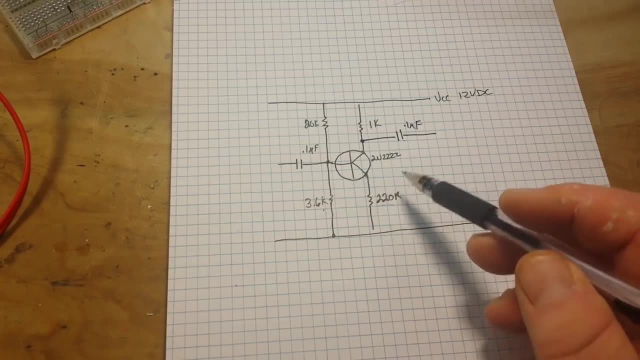 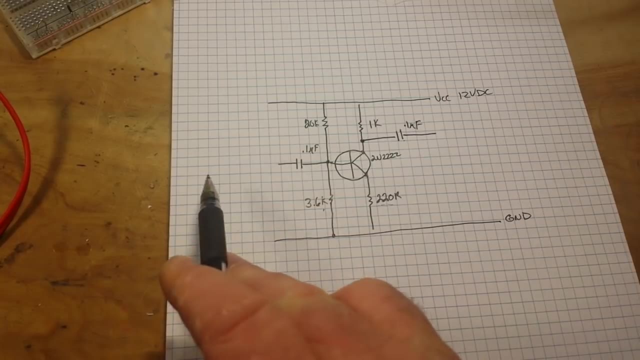 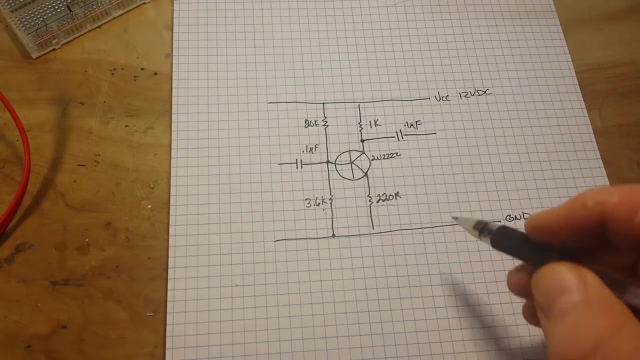 is right here in the amplifier and the reason for that is so that we're only getting the ac, the audio signal, audio signal in audio signal, out. we're not adding any dc to bias our circuit one way or another. and finally we're going to add one more capacitor here. 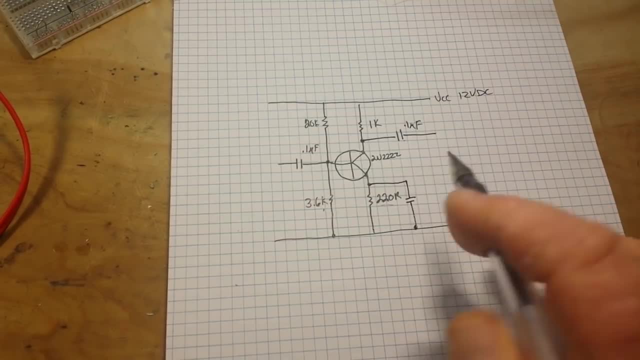 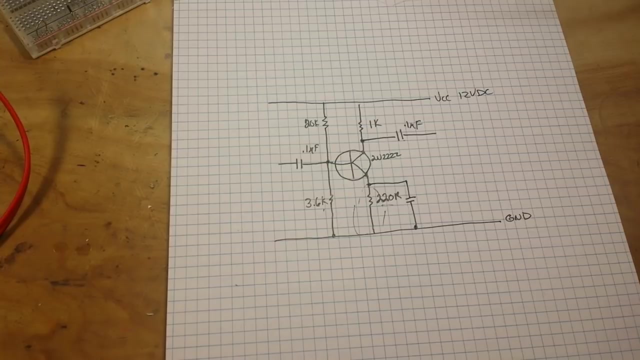 and that's going to do a couple things. it's going to bypass any hum which you can get from your mains if you're driving this off a power supply or anything like that, and it's just going to help to keep this thermal runaway from happening here. so there's our circuit, pretty simple. 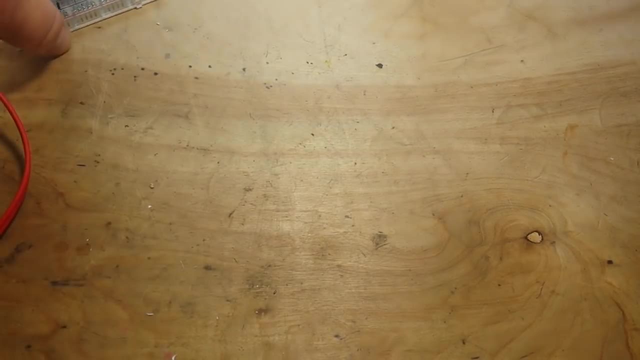 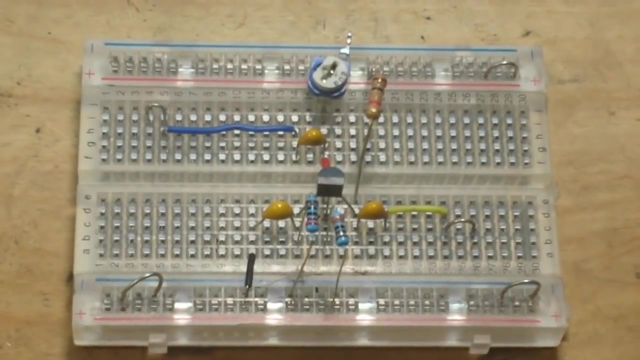 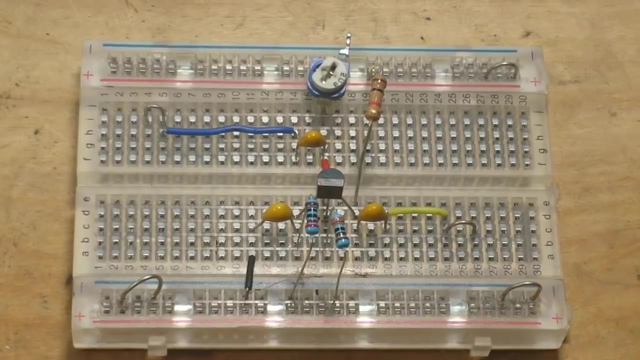 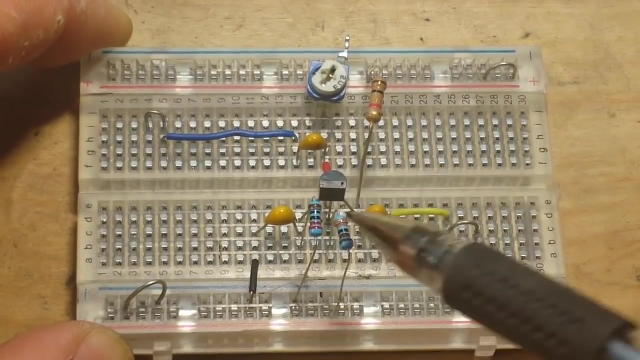 this is a class a amplifier, which means it is on all the time. which means, number one, it's going to be the most linear type of amplifier, which is good for audio, but number two, it is the least efficient type of amplifier. so here is our 2n 22, 22 transistor, and the pins from left to right are: 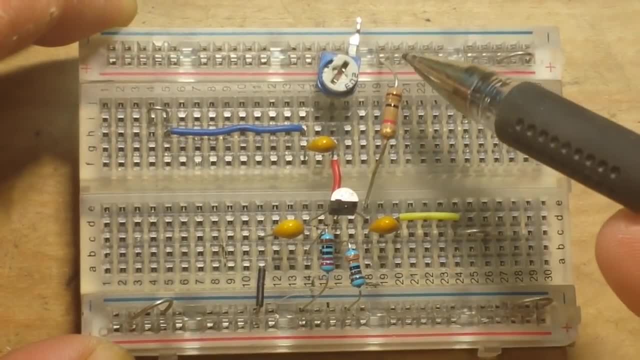 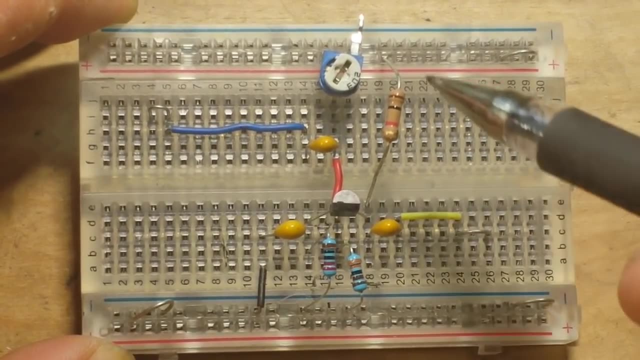 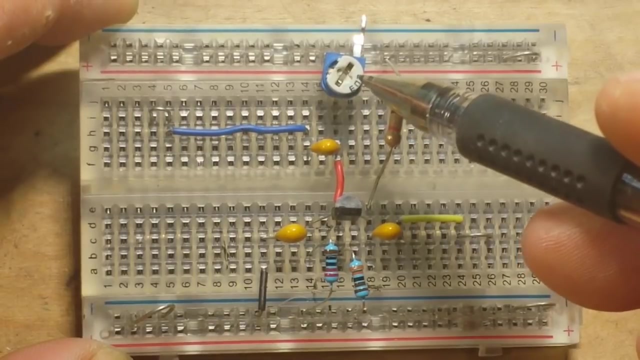 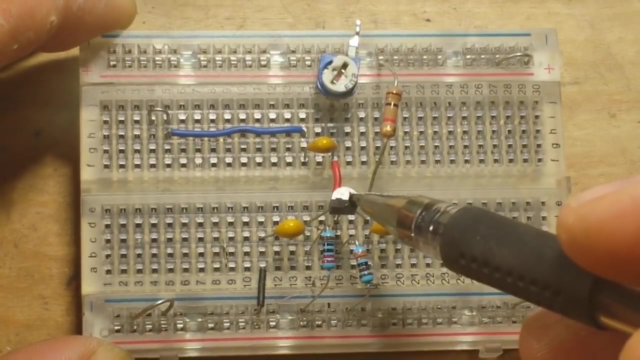 emitter, base and collector. here is our 1k collector resistor. coming down to our collector now, i didn't have a 20k resistor, so i'm using a 20k pot and i'm just using the inner leg and the wiper. so there's our 20k pot there and there's our 3.6k here, giving us our voltage divider. 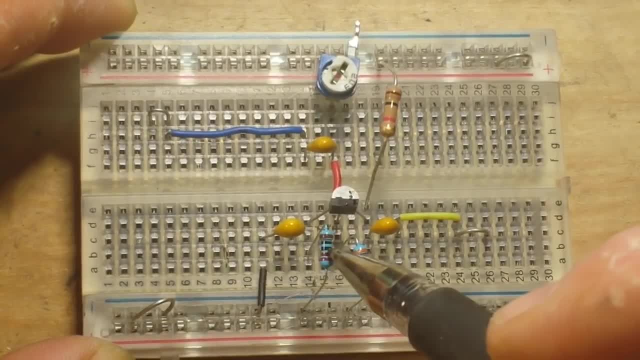 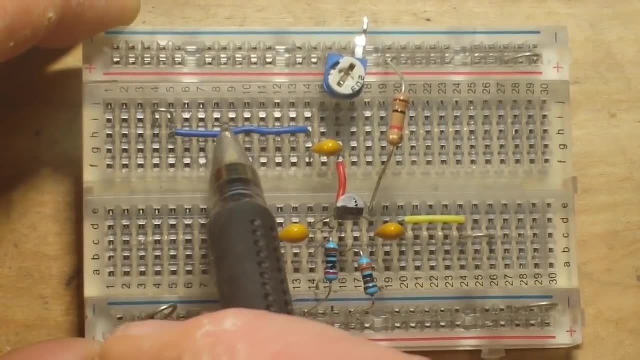 there's our emitter, there's our 220k or 220 ohm emitter resistor, and then let's look at our input. our input's coming right here into the base through this blue line and it's being decoupled there. our output is right here, the yellow. 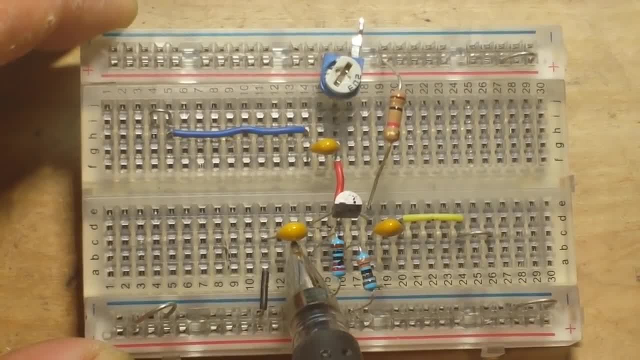 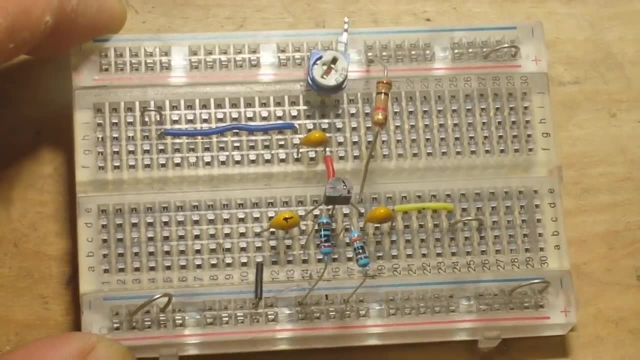 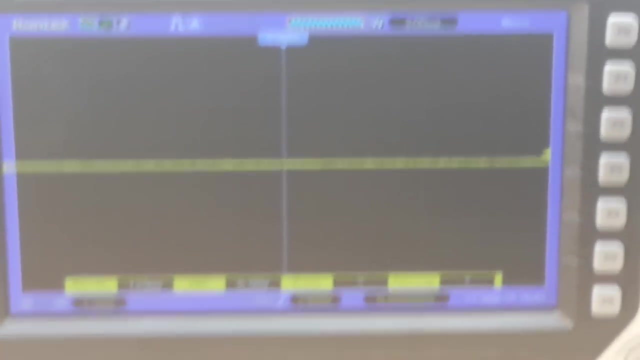 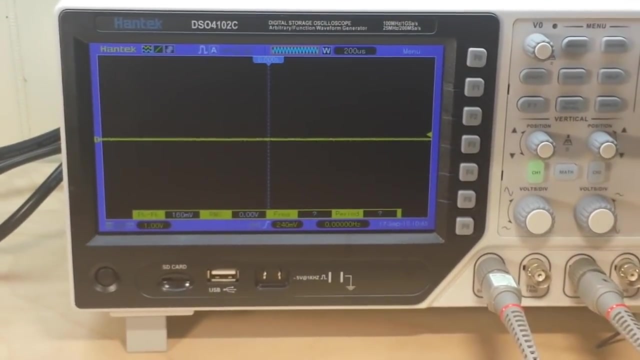 line and it's being decoupled there and finally we have this last emitter capacitor right here going to ground. so there's our circuit. now let's set up our test. yeah, zoom out here just a little now. if i bring up the signal generator, you can see we have it. 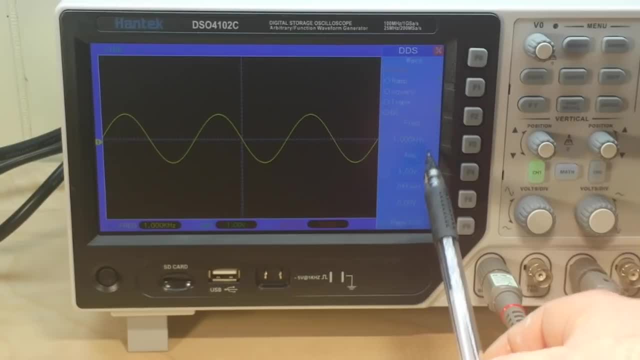 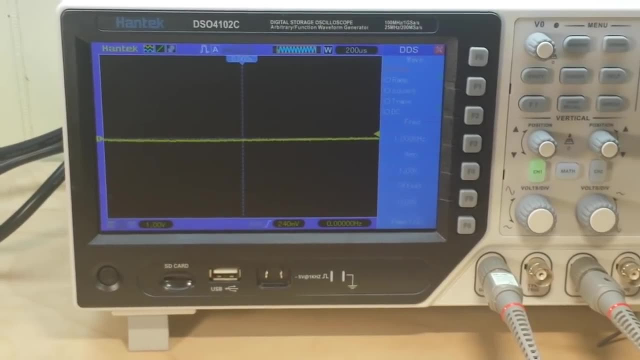 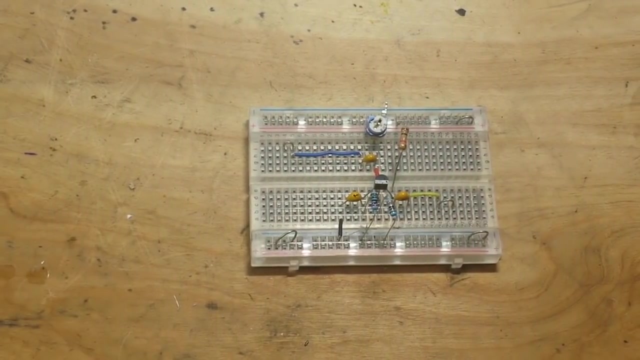 yeah, zoom out here just a little now. if i bring up the signal generator, you can see we have it set for a sine wave 1k and one volt going in, so let's hook it up. we're going to start by feeding our circuit with the 12 volt dc. 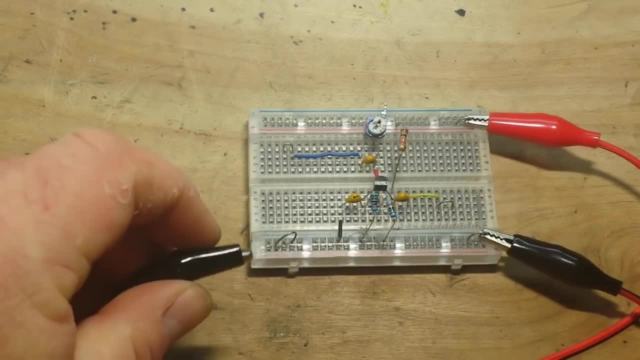 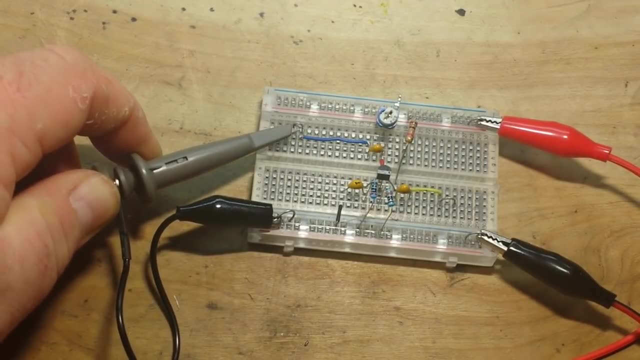 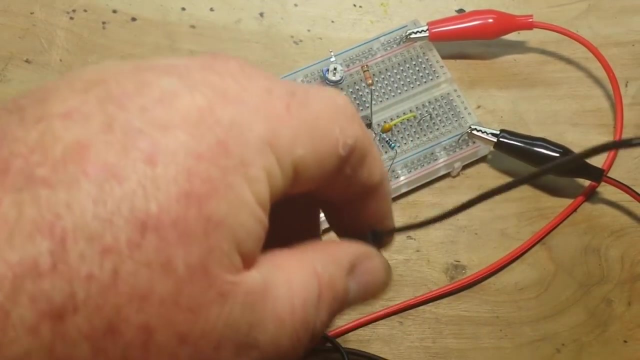 and then we're going to inject the signal, always hooking up my grounds first. so the signal from the signal generator, the one volt 1k sine wave, is going in there, and what we can do here is: we'll take a look at it on the scope. 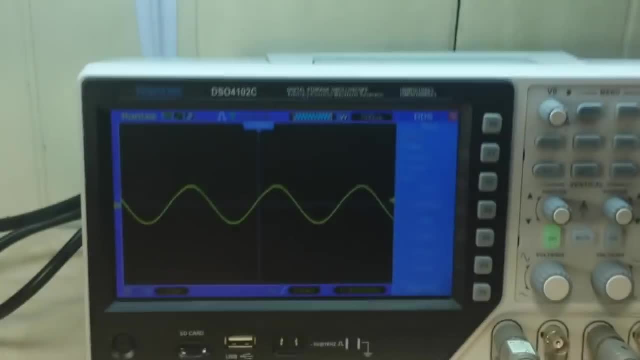 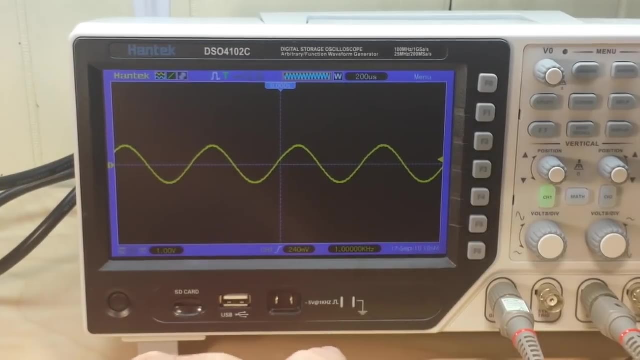 okay, so we're hooked up there. okay, so we're hooked up there. there, we're going to get rid of that screen. all right, so we are seeing a one kilo. all right, so we are seeing a one kilo. we're at one volt per division. 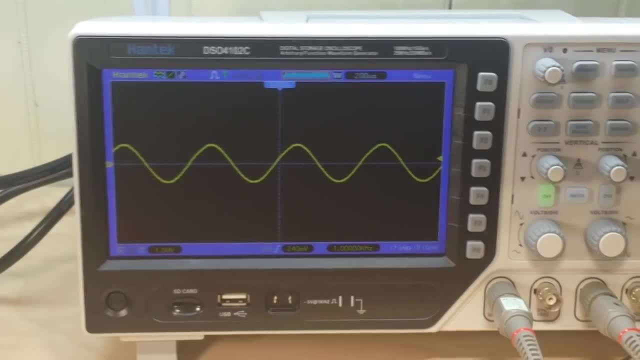 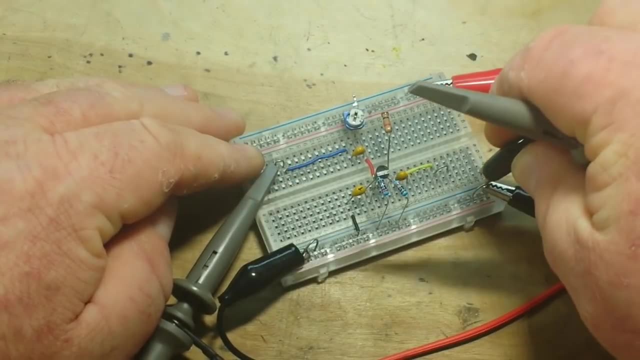 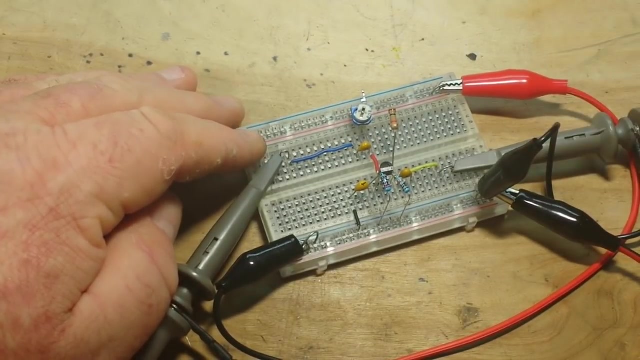 we're at one volt per division, so we're seeing two volts peak to peak. that's our input. now let's switch it over here to the now let's switch it over here to the output of our circuit. and take a look at that. and take a look at that. 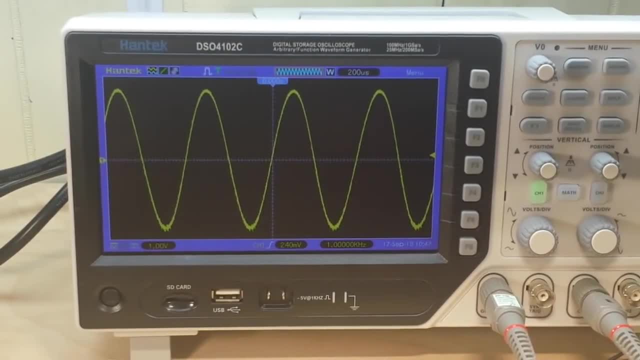 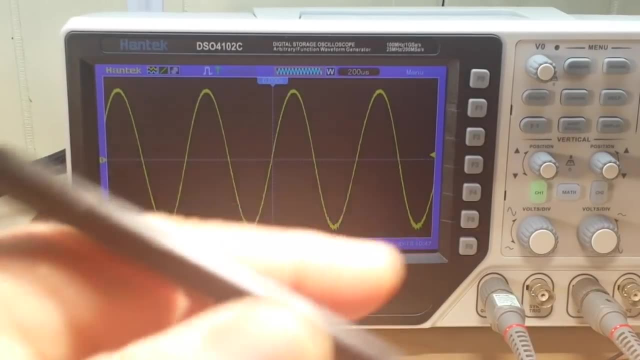 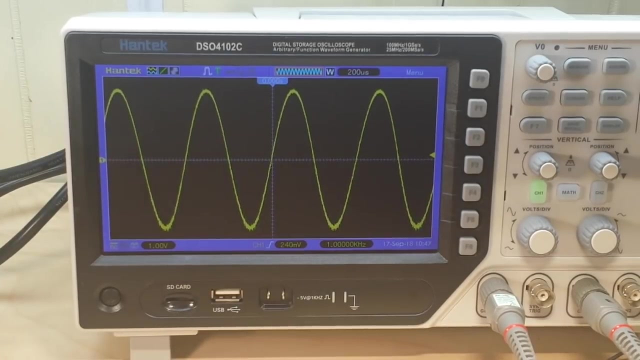 there we go again. now we're seeing our output to our circuit. so we're at one volt per division there and we are one, two, three and a half divisions. we bring up our measure, we can see: there's our frequency, there's our mean and there is. 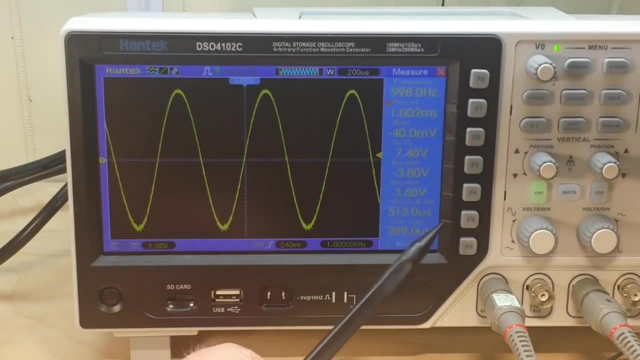 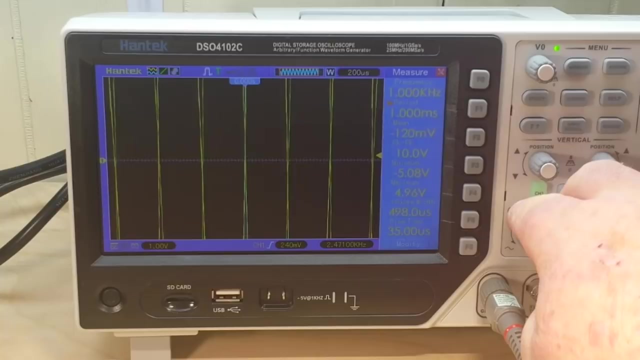 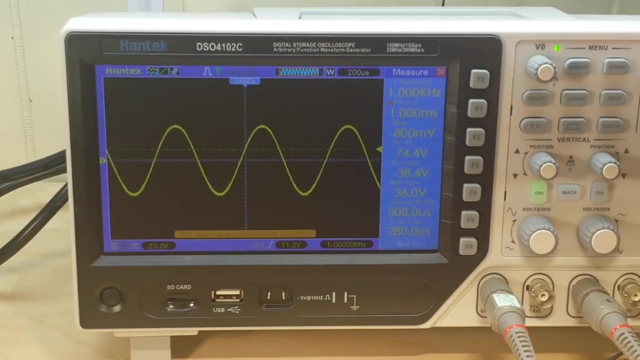 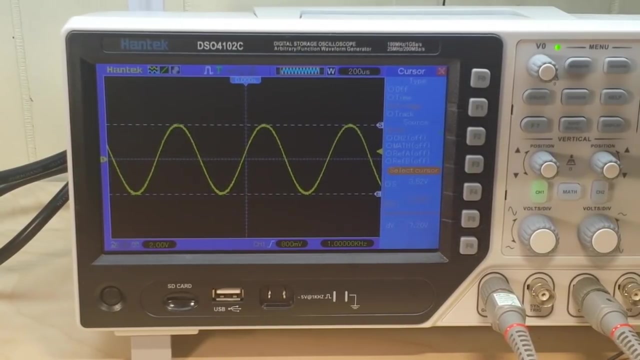 our peak to peak. why is our peak to peak say minus 40 millivolts? because my dumb butt had things set up wrong. I'm losing my mind here. give me a second, okay? well, I had the x 10 attenuator on there, so that was our problem. anyway, I put on the cursors here so we can. 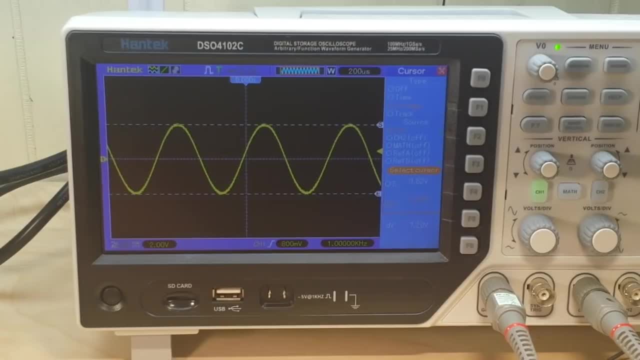 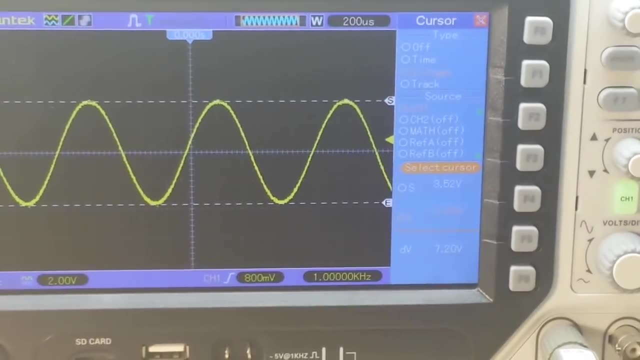 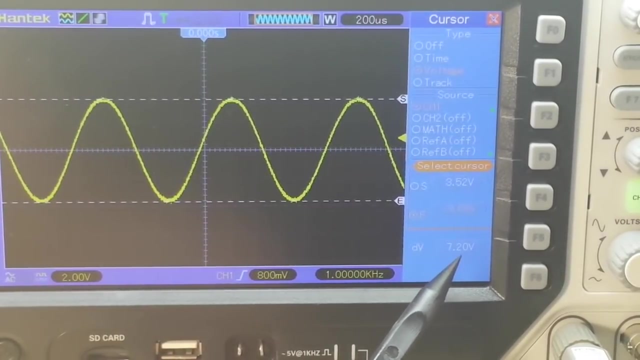 measure it and zoom in there and get you a better view so you can see what's actually going on. there we go. so our two volt peak to peak that we're with. one volt peak to peak that we fed in is now seven point two volts peak to peak and 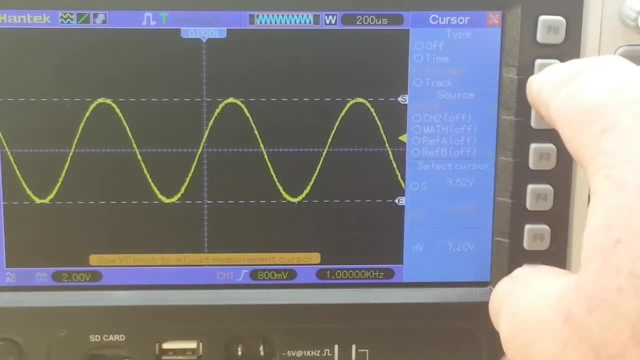 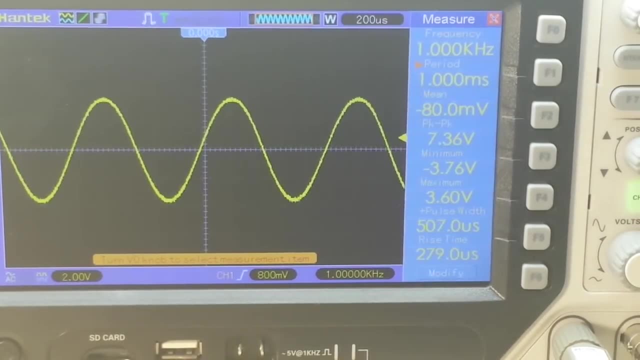 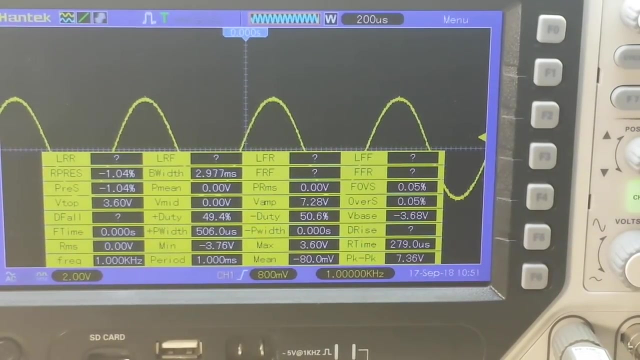 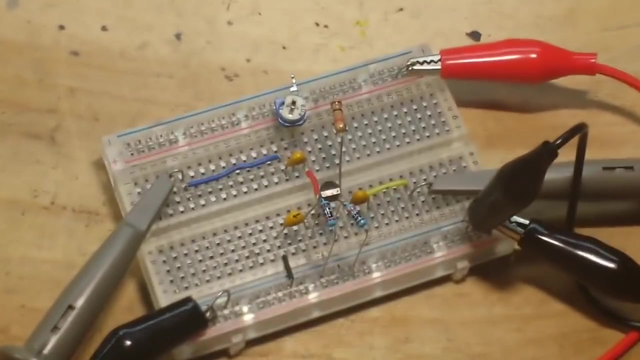 then we're at zero, and we're at zero and this is our common emitter amplifier. I hope that helps to explain things a little bit better for you and give you an idea of how you can build one yourself. it's not that hard. I'm still getting used to this new scope. I'm going to measure there we go. so that is our 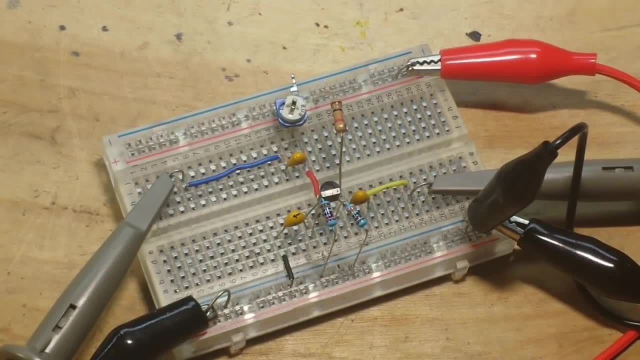 common emitter amplifier. It's a lot of fun and it can be pretty useful to do. Alright, if you guys enjoyed this, give me a thumbs up, Feel free to comment and share, and don't forget to subscribe. Big thanks to all my patrons. 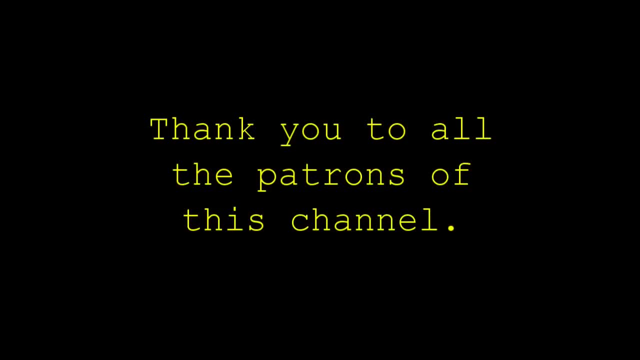 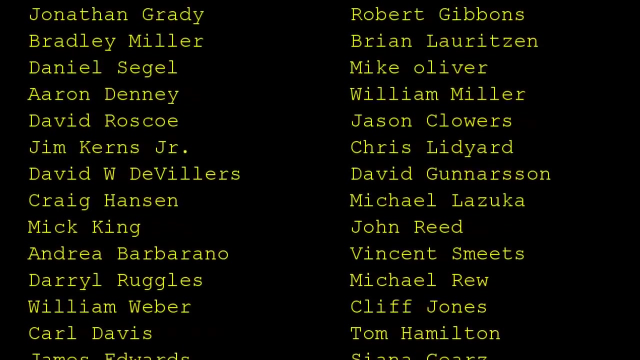 That's it. I'm out, Peace. Thanks for watching. 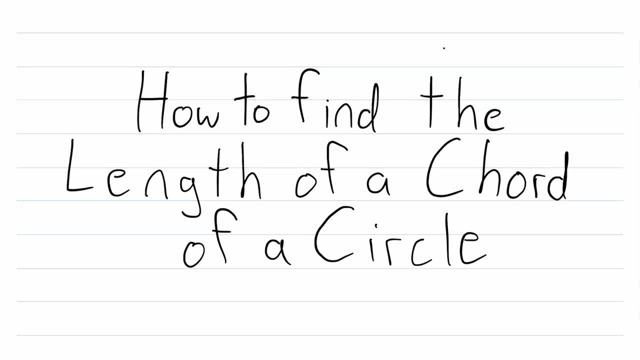 Hey everyone, welcome back to Wrath of Math. In today's video we'll be going over how to find the length of a chord of a circle. Recently I saw a math lesson with a bunch of nature sounds in the background. so just for a change of pace, I'll give you some. 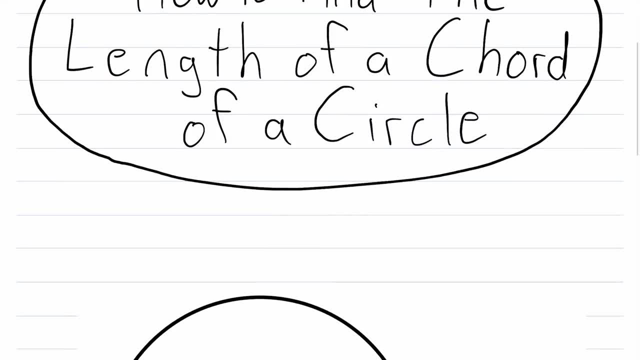 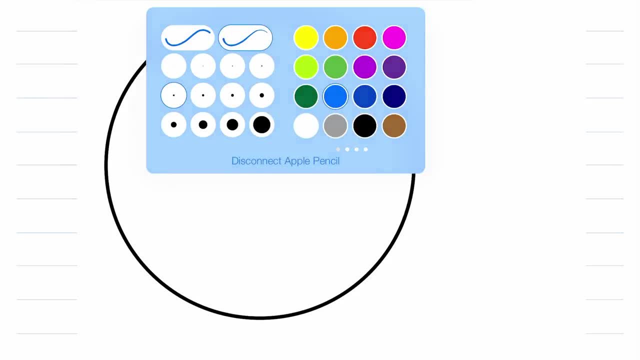 nature sounds to listen to today. So soothing, Just relax. listen to the birds. We're out in the forest scribbling in the dirt doing geometry. If I focus on the sound of the birds hard enough, I can almost drown out the rumbling of my stomach. So let's finish this lesson. 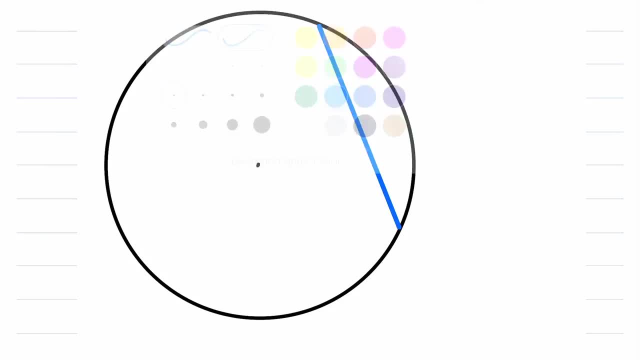 so that I can go eat Here. we have a chord of the circle. Remember that a chord is a line segment whose endpoints both lie on the circle. So that's great. This is a chord. How do we find its length? Well, there are really two key pieces of information that 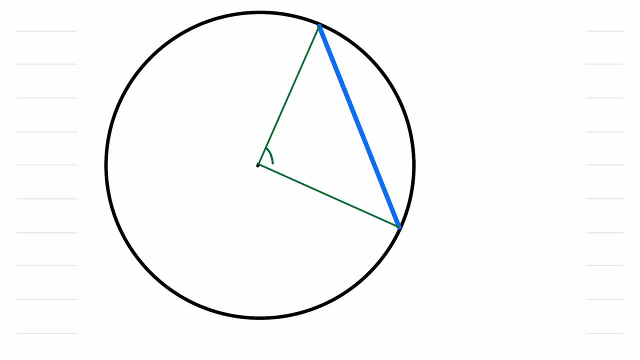 we need to know to find the length of this chord, We need to know the measure of the central angle subtended by the chord, That's this angle- here We'll call this angle theta- And we need to know the measure of the radius of the circle.